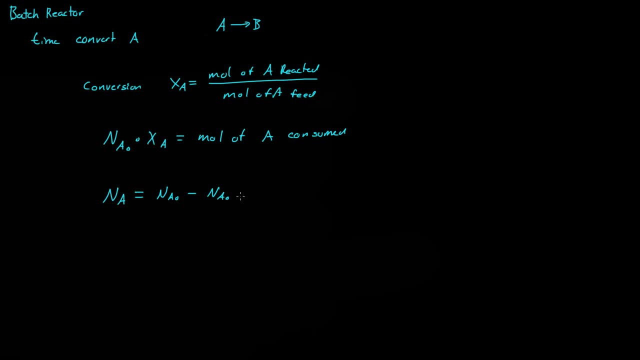 So then we get NA Not times XA. So this will give us the moles of A in the reactor at this time or at this conversion. So we actually haven't even gotten to the time. So if we wanted to convert 20%- 20% of the reaction- then XA would be 0.2. And then this would be 80% of whatever the initial amount of A was. So we can rewrite that as NA, not 1 minus XA. 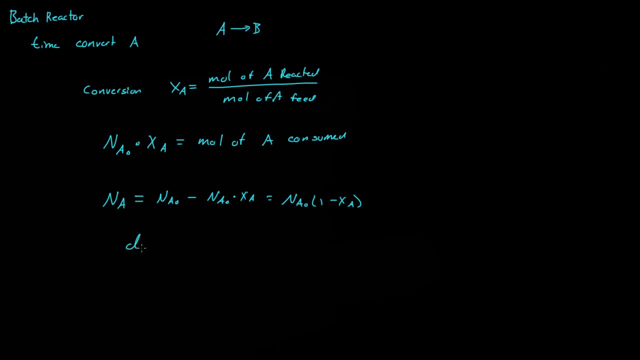 So that's another way of writing it. Now, if we wanted to know the change in the moles of A with respect to time, that's equal to the reaction rate of A times the volume. So remember, this is the change in the moles of A with respect to time and volume. the reaction rate is. So if we multiply that by the volume, we get DNA over DT. Now we're going to get that negative, or multiplying both by negative, 1.. 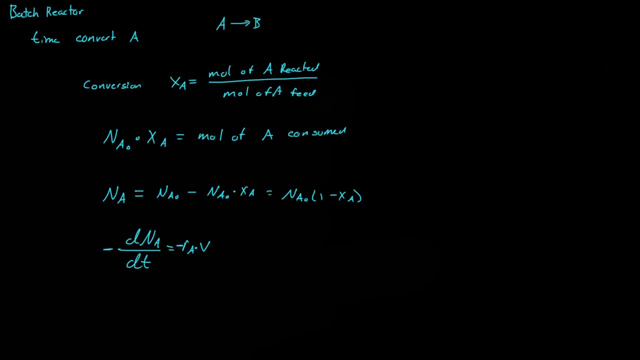 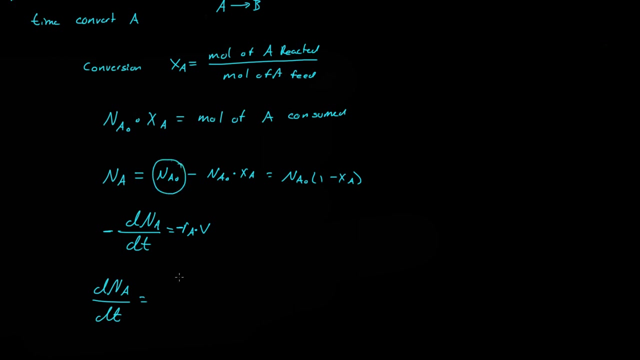 That's just to allow this to be a positive number. So if we do that and we then differentiate this equation, this equation, we get DNA all over. DT is equal to well, this is a constant, so that's 0.. 0 minus well, again, this is constant. so NA not. So if that's a constant, is XA a constant? No, XA changes with time. 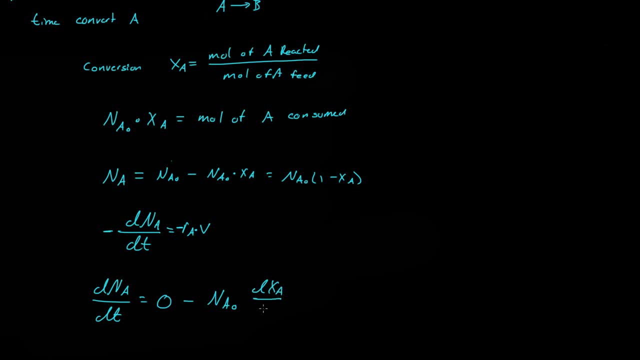 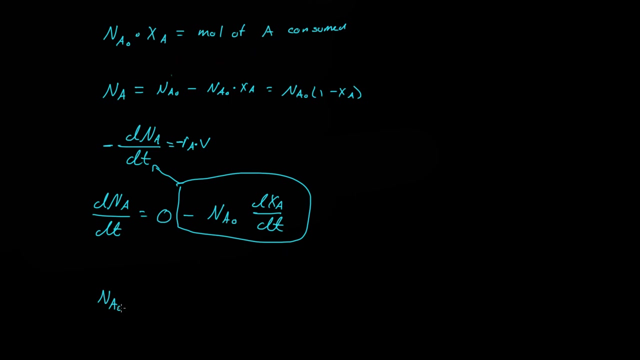 So then we have DXA all over DT, So now we can actually plug this part in for that. So we'll plug that right there And what we get is we get a positive NA or the initial amount of A in the reactor that we feed into the reactor times. DXA all over DT is equal to a negative reaction rate of A. 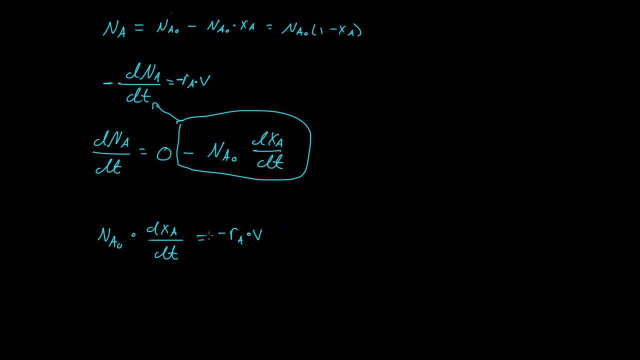 So we can write A times V and, with a little bit of rearrangement, we'll just multiply both sides by DT so we get: DT is equal to NA, not times DXA, all over a negative RAV. So all I did was divide this by RAV, this by RAV- a negative RAV, and multiply it by DT.